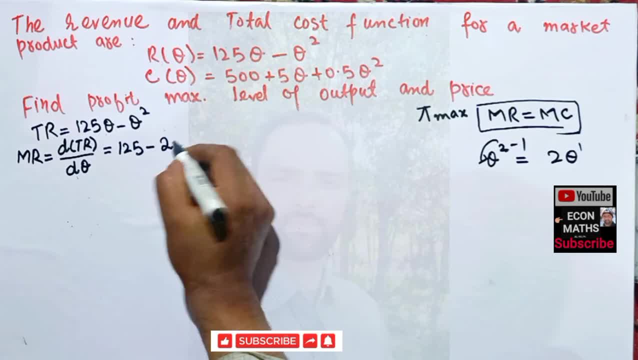 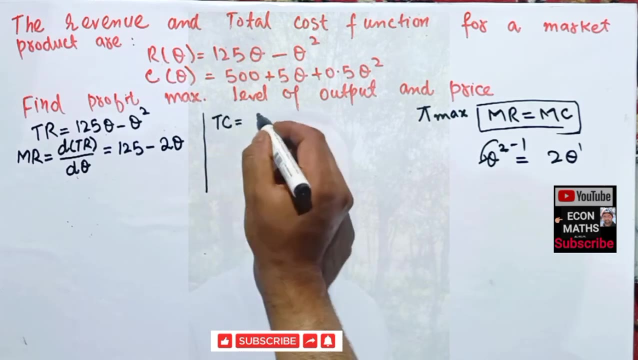 So 2 minus 1 is 1.. So here we have this: 2 Q. This is our marginal revenue. Similarly, we are being given the total cost function. That is, so I will write here: Total cost is given as 500 plus 5 Q plus 0.5 Q square. 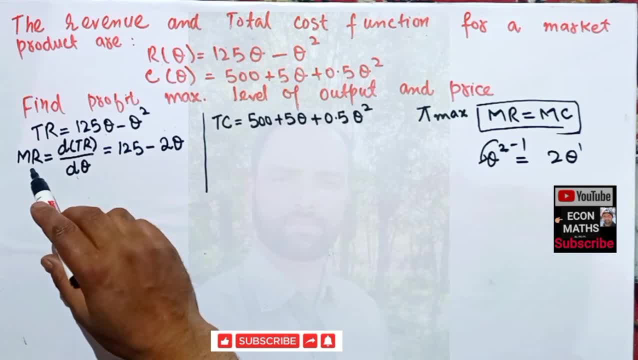 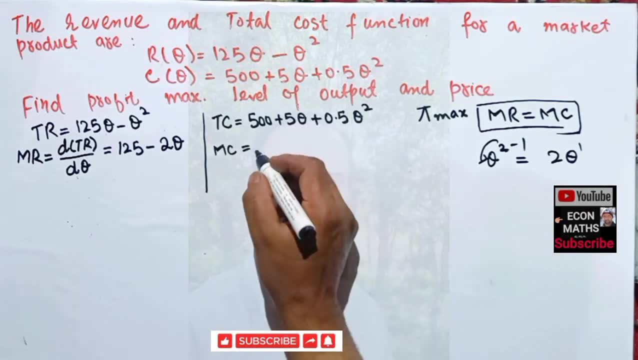 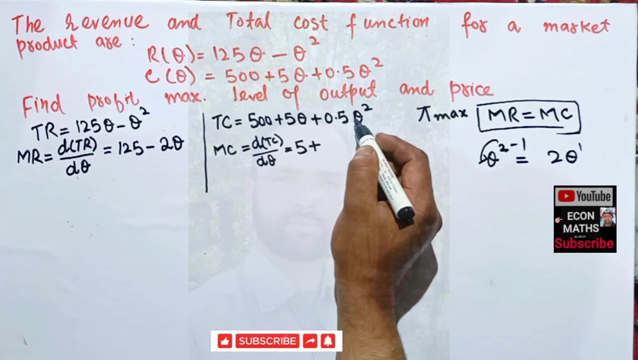 And total cost is like the total marginal revenue. So marginal revenue is the first derivative of total revenue. Similarly, marginal cost is the first derivative of total cost function with respect to quantity, That is, differentiating total cost function with respect to quantity. So derivative of constant is always 0.. The derivative of Q is 1.. So 5 into 1 is 5.. Plus, the derivative of Q square is 2 Q. Okay. So we have 2 into 0.5 Q square. 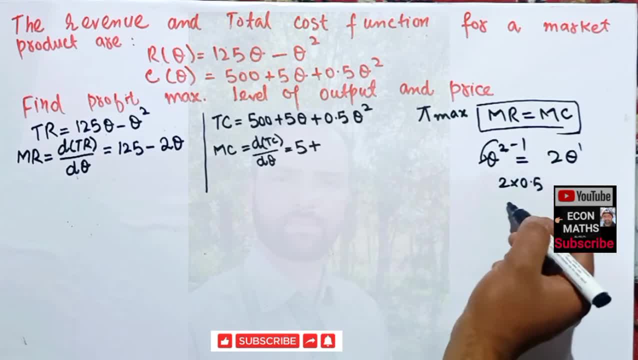 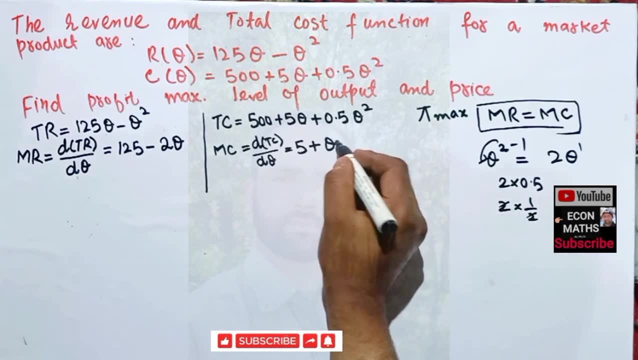 2 into 0.5, which is equal to 2 into 1 by 2.5, can be written as: So we get here only Q, So 0.5 Q square. The derivative of Q square was 2, Q And 2 into 0.5 is equal to 1.. Okay, This is our marginal cost, This is our marginal revenue. 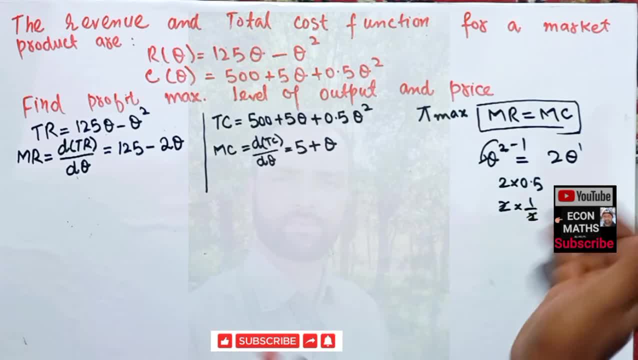 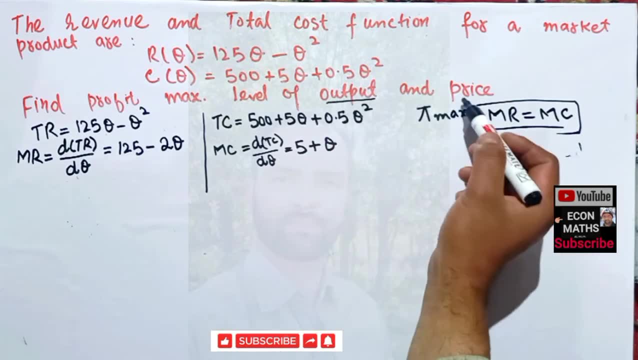 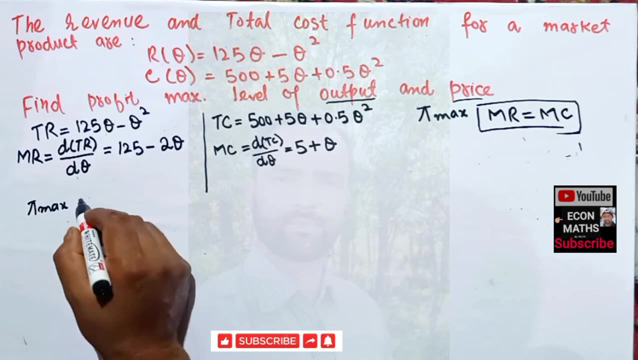 Now, coming to the solution part, find the level of output and price first. we will find the level of output now. profit maximization condition is rather the first order condition. we have two conditions for profit maximization, okay. so first order condition is that our marginal revenue should be equal to marginal cost. so marginal revenue is 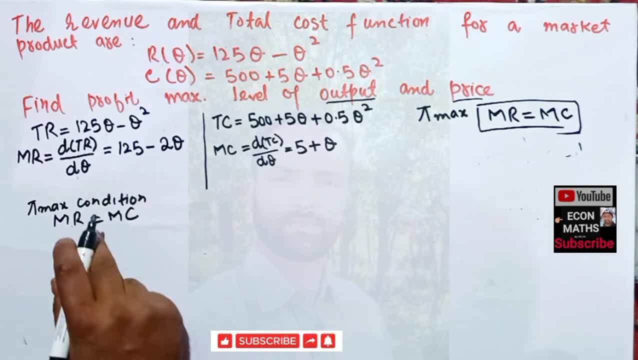 this 125. so I write: this is 125 minus 2 Q should be equal to marginal cost, which we have calculated. that is 5 plus Q and we can transpose this for you on LHS. this will become 125 negative 5, similarly transposing negative 2 Q on our HS. so this will: 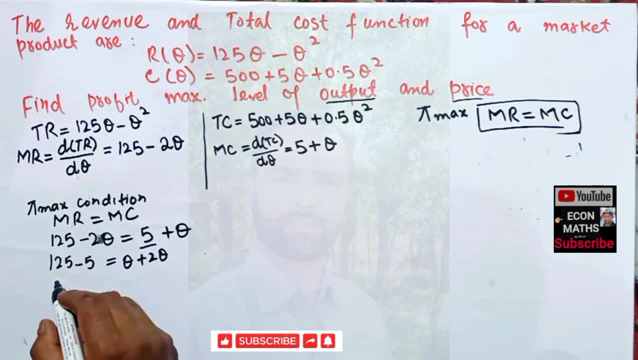 become positive: 2 Q, 125 minus 5 is equal to 120, and we have Q plus 2, Q is equal to 3, Q or our Q is equal to 120 divided by 3, which comes out to be three. ones are three, fours are 12 and we have three. zeros are zero. so equilibrium level of: 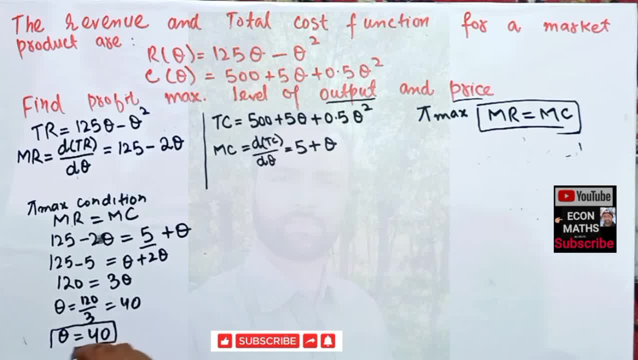 output is 40. okay, so we got the profit maximizing level of output. that is equal to Q, that is equal to 40. sorry. now coming to the next part of the question, that is, we have to find the price. okay for that. what will we do? I will write. 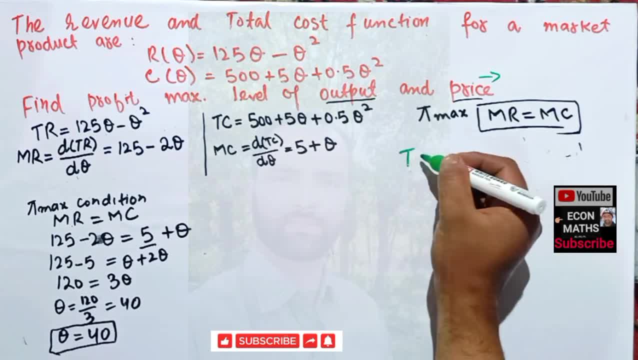 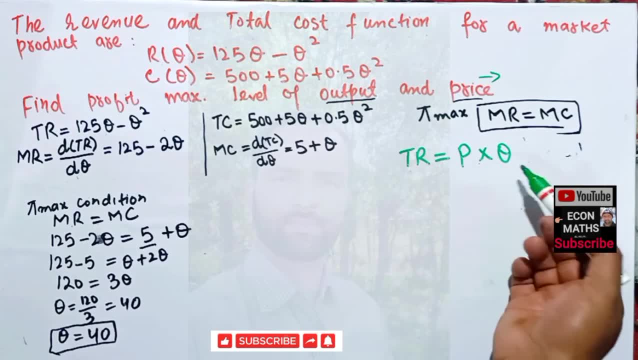 here. we know that total revenue, total revenue, is equal to price into quantity. this is the relationship between. when we multiply price and quantity, we get the total revenue. okay, now our total revenue is given. so I will right here: total revenue is given, that is 125 you Q minus Q square. this is our. 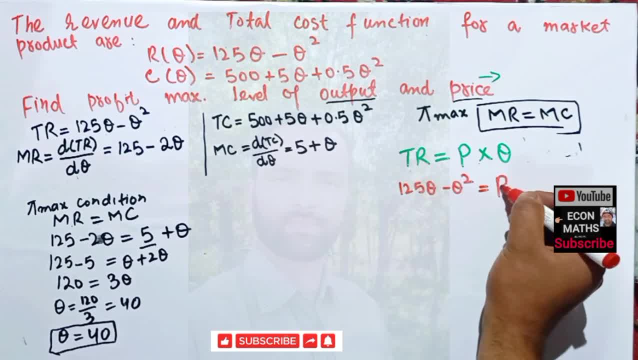 total revenue, which is equal to price times Q. okay, Now what we can do here. we can transpose this Q on this side, Since it is multiplied here on the RHS side. when we transpose, it will get divided to each of these two terms. okay, 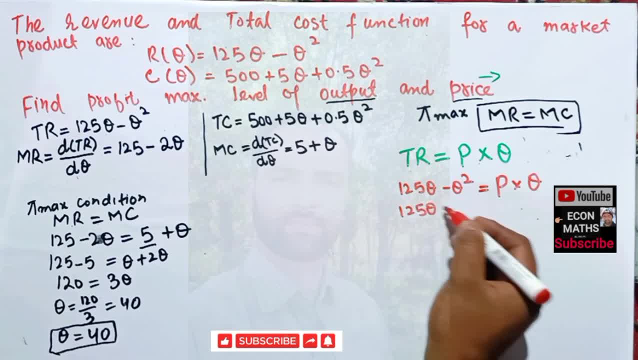 Or we can write: 125Q minus Q squared is equal to P divided by Q. So because since on RHS it is in the multiplication, when transposing it will become the denominator, okay. Or we can write it here: 125Q divided by Q minus Q squared divided by Q, okay. 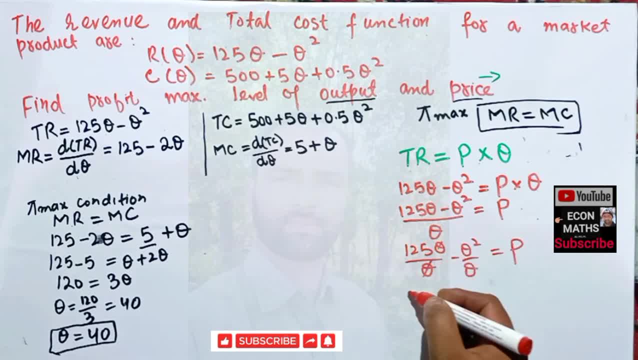 Which is equal to P. Now Q and Q will get cancelled. We have 125 minus here. 1Q will get cancelled. We are left with only 1Q here, which is equal to P. That means our inverse demand function would be like this: 125 minus Q.